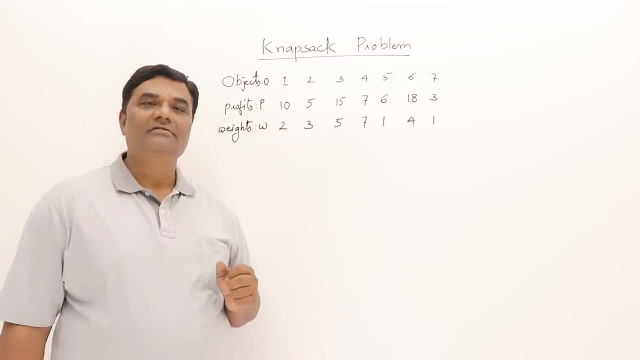 And every object is having some weight. So objects are there, Every object is having some profit and every object is having weight. Okay, weight, we understand. What is this profit? See, there is a bag given here. That bag is called as knapsack. The bag capacity is 15.. These are seven objects. Bag capacity is 15.. There is a bag whose capacity is 15.. Let us say kg. 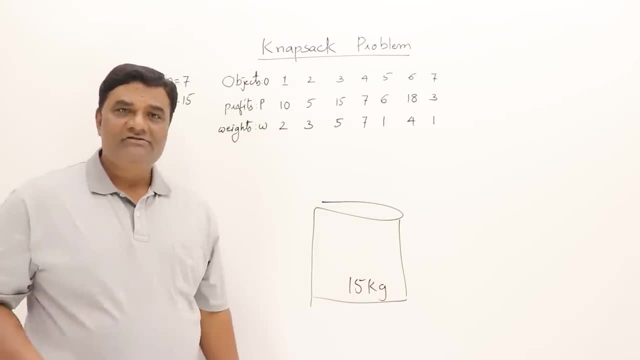 Okay, it can be kgs also, pond also, it can be anything. So I am assuming it as kg. Now what we have to do is we have to fill this bag with these objects And we will carry this bag to a different place and we will sell away these objects. We get that profit. So that profit is the gain that you get by transferring these objects to a different place. 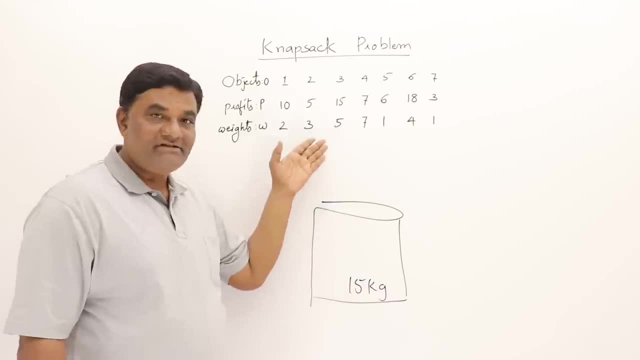 So for transferring you have to carry them in this container or bag. So I can also call this knapsack as container. This is a bag or knapsack. I can also call it as container. So the problem is a container loading problem. So we find this type of problems in daily life. A lot of goods are transported daily from one place to another place. Now the problem is about filling of that container with the objects. 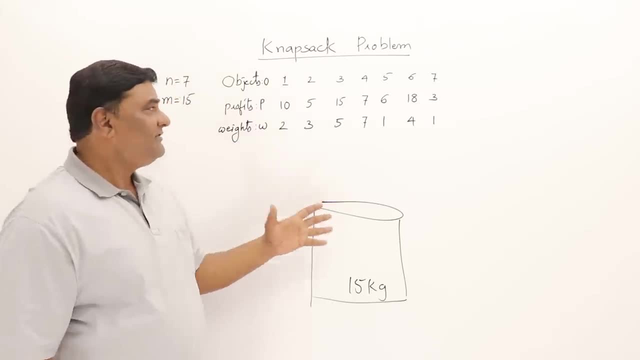 When it becomes a problem. If you have the objects whose total weight is more than the capacity of the container or a bag. If you have less, all can fit in, then no problem at all. If you have the objects more in number, their weight is greater than the capacity of a bag, Then it is a problem. So already we have some objects here, So I have to fill this bag with these objects such that the profit is major. 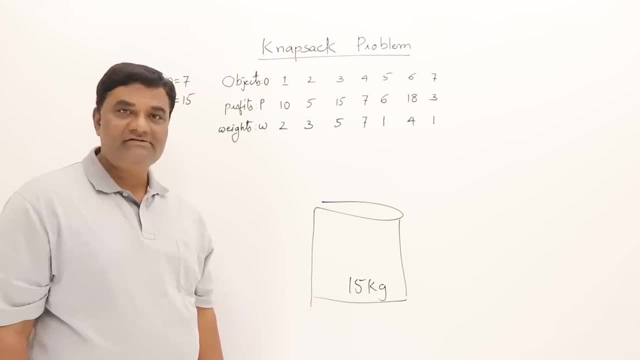 Maximized, Profit is maximized. So this is a optimization problem And it is a maximization problem. Maximization problem: Can we follow greedy method? Yes, we can follow greedy method on optimization problem if it is suitable. Next thing, What is the constraint here? The total objects included here in the bag. their total weight should be less than or equal to 15 kg. 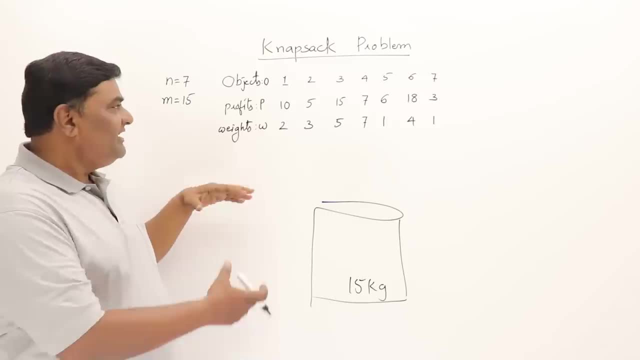 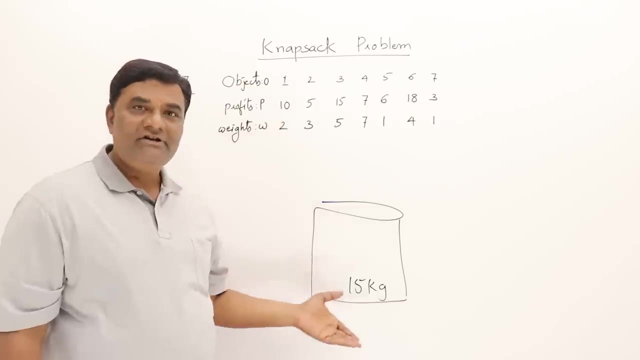 This is a constraint, So I can give various solutions. I can say that just put only one object and take it. It's not maximum. I'll say all, All cannot fit in, It's not feasible, So it cannot be optimal. So there can be many solutions. You can say: take this, that and all and fill this one, But we want maximum result. That's it For a problem. there can be many solutions, But those solutions which are giving the solution which is giving maximum result is an optimal solution. 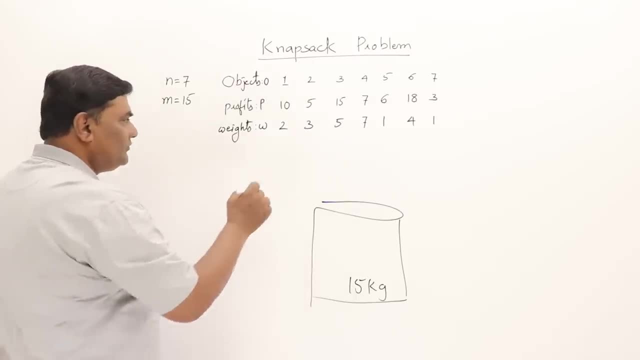 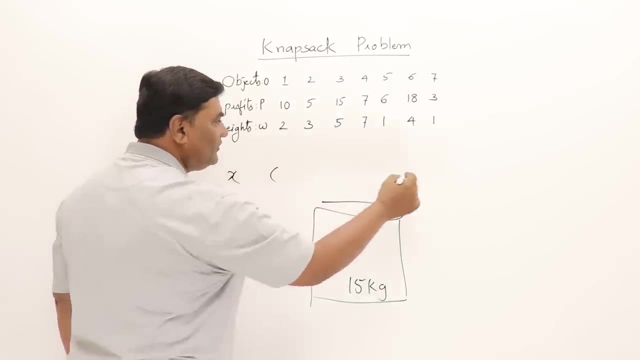 Let us see how to solve this one. See, what I am going to do is for these objects. I am going to include them. So I will write down whether the object is going to be included or not included, or how much it is included. I will write down here x values. So here I will be writing x1 or x2 or x3.. Right, X values I will be writing. So this x value can be either 0 to 1.. This x can be from 0 to 1.. 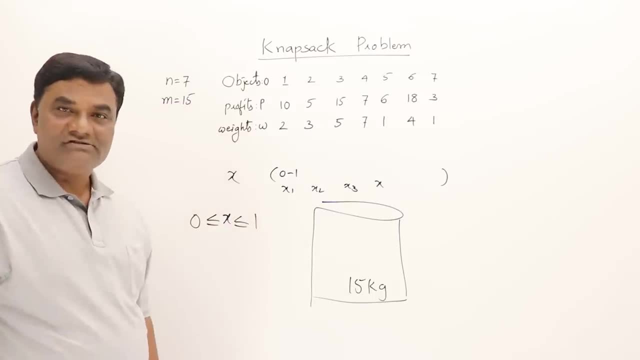 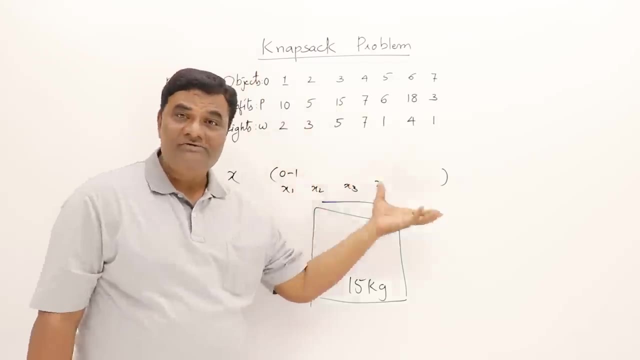 So it means I can also take fractions. Yes, So now listen one thing very carefully. This knapsack problem is for those objects which are divisible. I have something of 5 kg means I need not take all 5 kg, I can just take 2 kg also, 1 kg also, So these objects can be divided. So what type of objects? If I take an example, these may be divided. 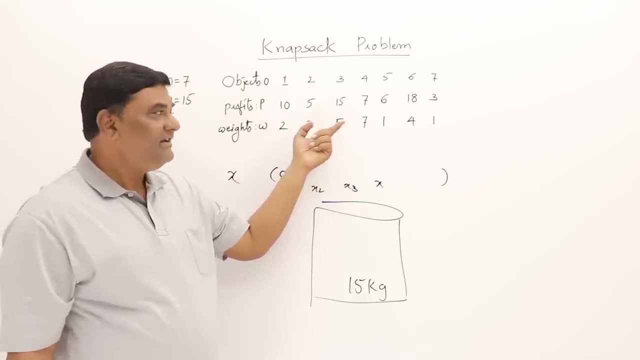 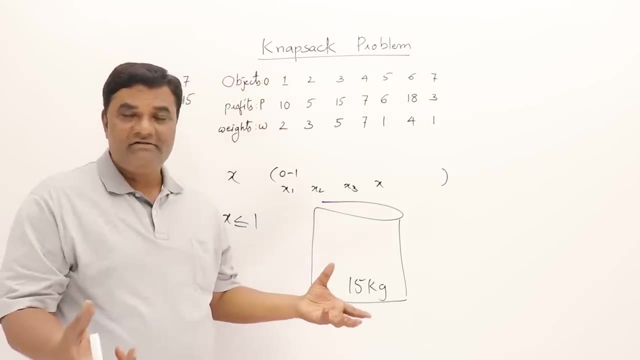 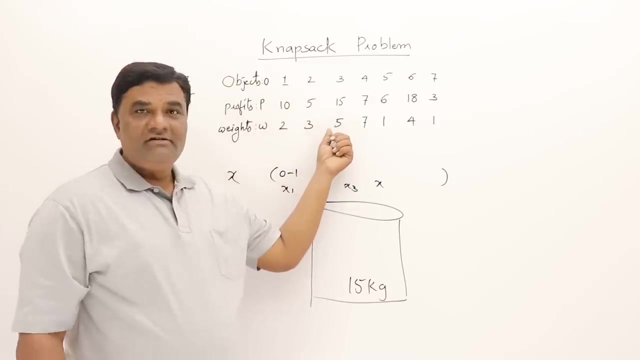 Vegetables: 7 kg of potatoes, 5 kg of tomatoes, Something. So instead of taking 5 kg I can take 2 kg. also Means, it can be divided. Yes, So this is not about those objects which are indivisible. Let us say, 5 kg grinder, mixer, 7 kg washing machine. It cannot be divided, It cannot take half of that washing machine, So I have to take the full one. So here I can take the fraction of. 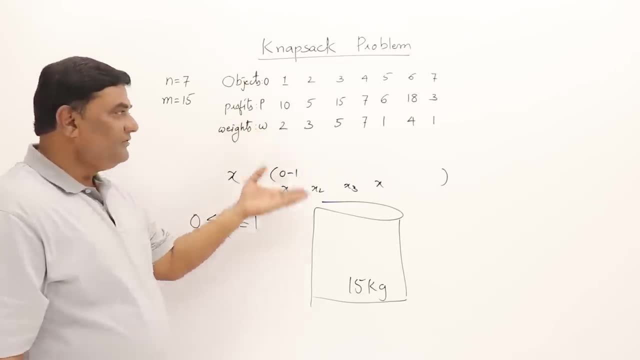 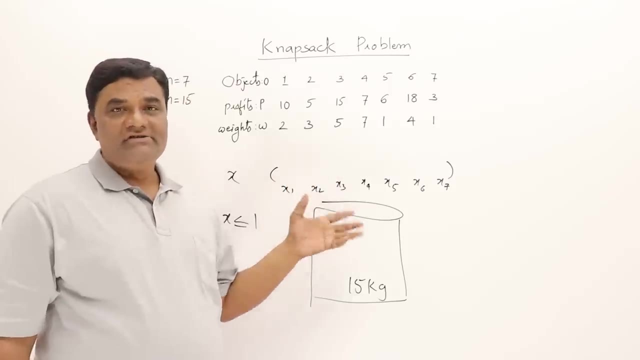 an object also. So that's all. Whatever I am including, that can be a fraction starting from 0 to 1.. Now let us see how to include these objects in the back. What should be my criteria method for including them in the back? You may be saying that this is giving highest profit. Take that one first. Yes, that is giving highest profit. Take that one first. But 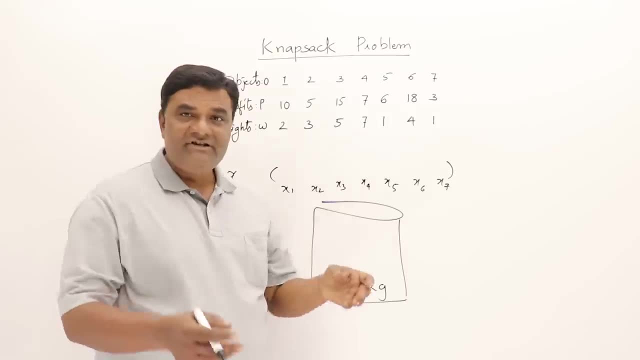 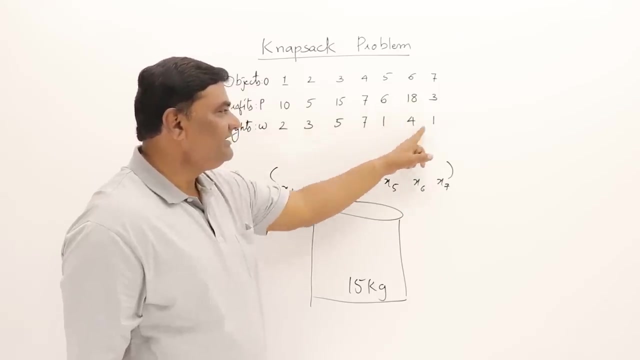 I can say that first fill the bag with smaller things so that I can get more and more things in the bag and I can make more profit. More things you carry, more will be the profit. So I prefer, take these objects first with one 1 kg weight or smaller weights. So your idea is also good: Take the maximum profit one and my idea is also good: Take the smaller weights one so that I can have more objects. 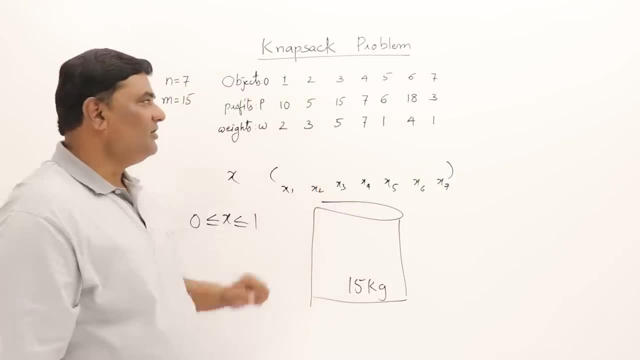 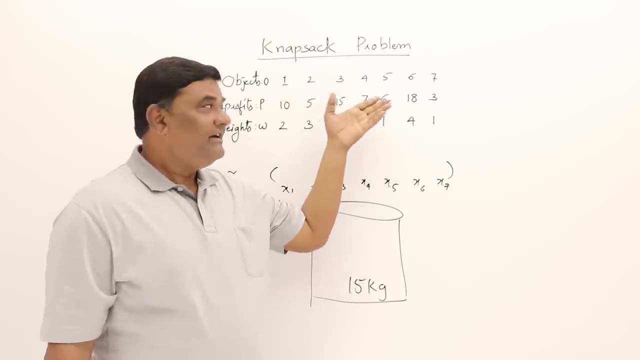 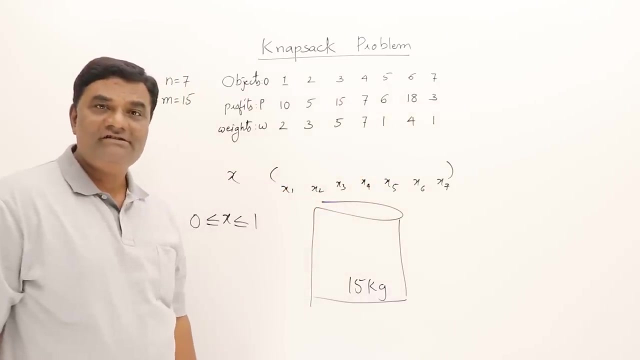 But what is the right method? I shouldn't select the objects. which is having highest profit by weight is 18 is the profit. So I say that 18 bucks is the profit. then that profit is for 4 kg. It's not for one kg, It's for 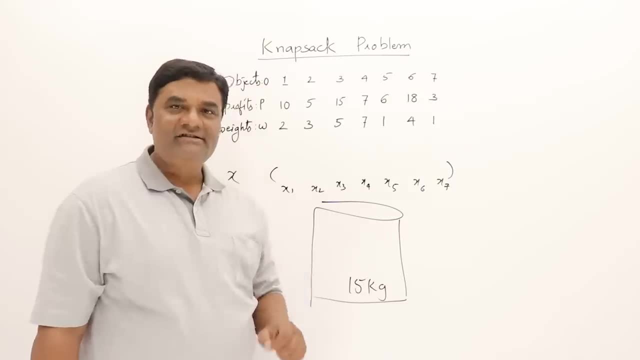 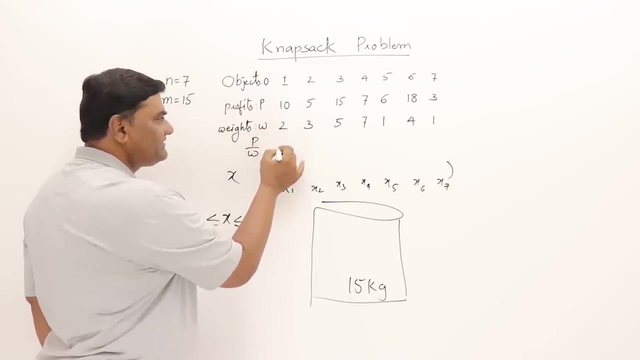 4 kg. so how much? So that's it? We should select the objects who are having highest profit by weight, by per kg. whoever is highest, that I should take. So I should calculate this one, So I will calculate profit by weight for all these objects. So this is 5. 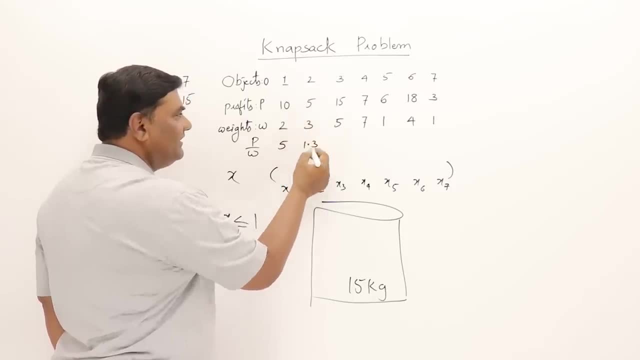 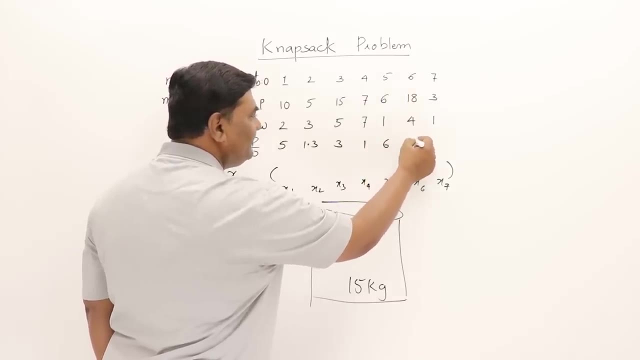 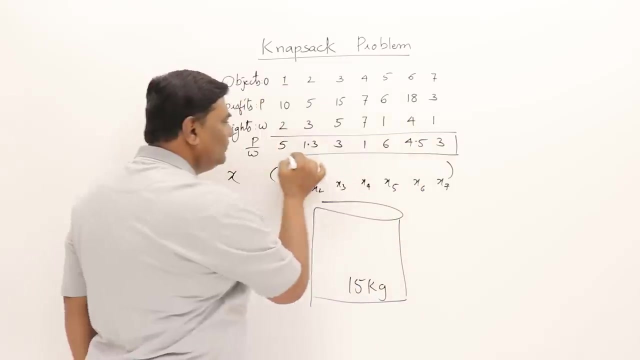 and this is 1.3 and this will be 3.. This is 1 and this is 6, and 18 by 4 is 4.5 and this is 3.. Now I have these profits and weights of all those objects. Yes, this is the right selection procedure. 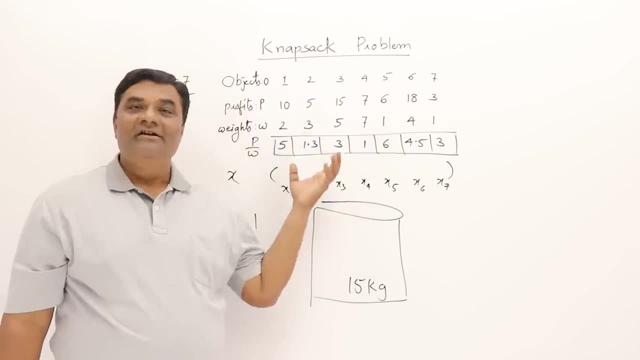 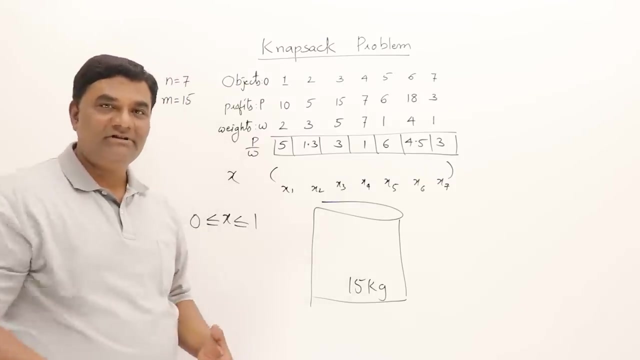 for the object. So the object should be selected based on their profit by weight. So the one who is having highest profit by weight that I should put it in the back first. All right now. this is the greedy method. Let us see what the greedy method is. 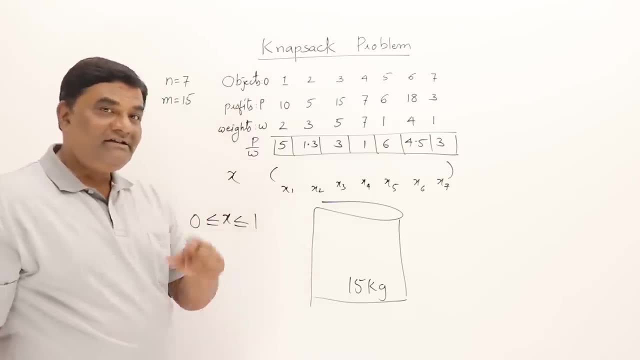 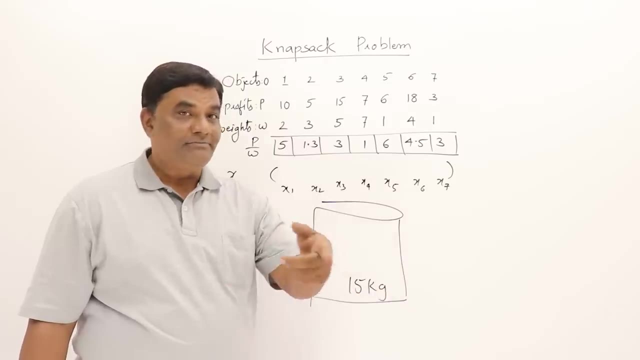 I was explaining you the problem so far. Then I said on what basis I should select this. Now we decided that we will select the object based on their profit by weight. This is our procedure Now. greedy method says that first you decide how you are going to select the input, Then go on. 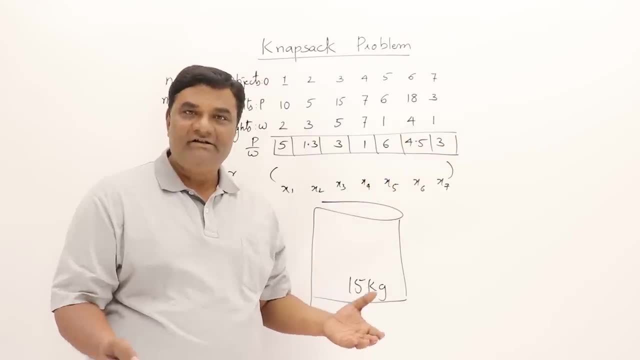 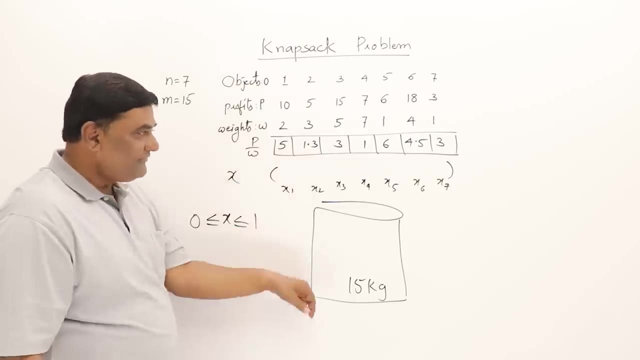 selecting the input one by one. So we already selected the method. We are going to select them by profit by weight. Now we will be going on including them one by one. So which object I should include first in the bag? The highest profit by weight. that is fifth object. So I 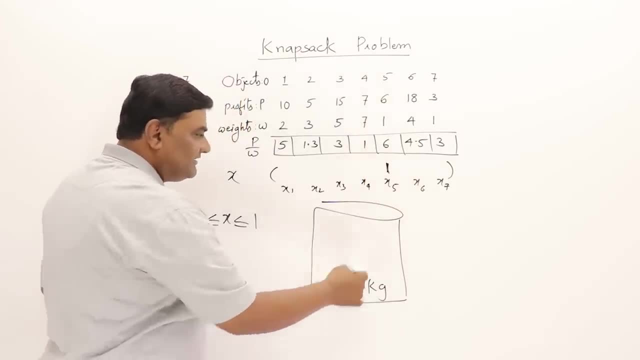 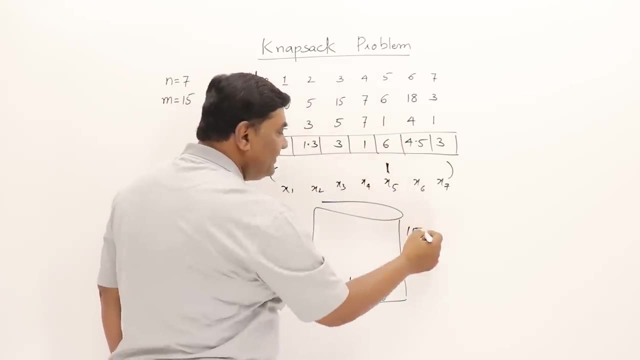 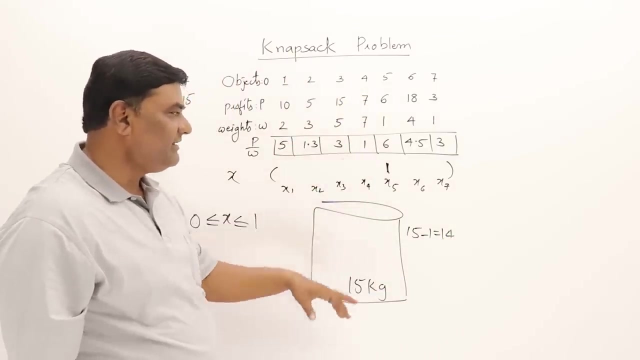 will include this whole thing. So now this is: this is 15 kg, right? So 15 minus how many kg? this profit, this object is one. So now remaining 14 kgs I have. So I have included that sixth of fifth object in the bag and I got the full profit six. Now who is next? This one, I will select this one. 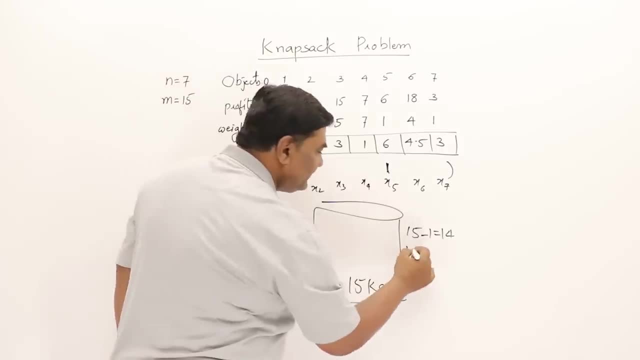 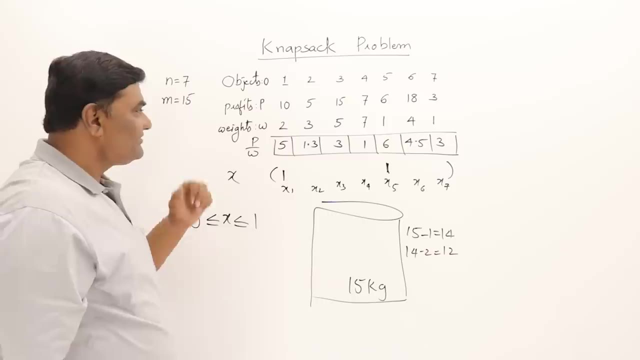 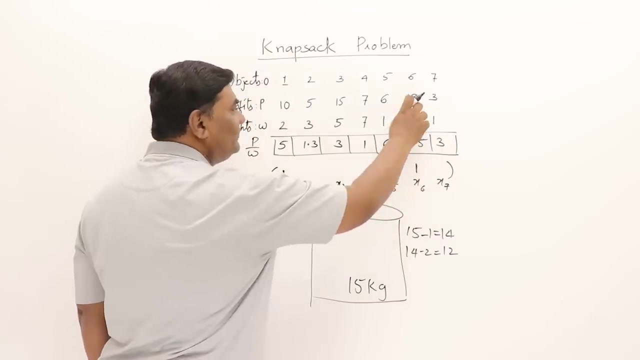 also this whole, all two kgs I will take. So this is 14 minus two kgs. Now I have dual kgs Remaining in the bag Now, which is the next object. So this is the highest. then this is the next highest. This is the third highest. I will select this object also completely full, So full. 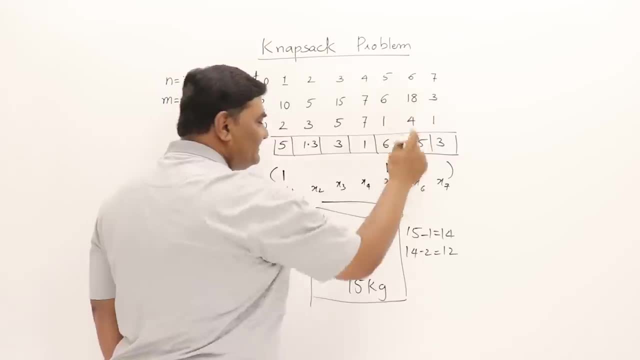 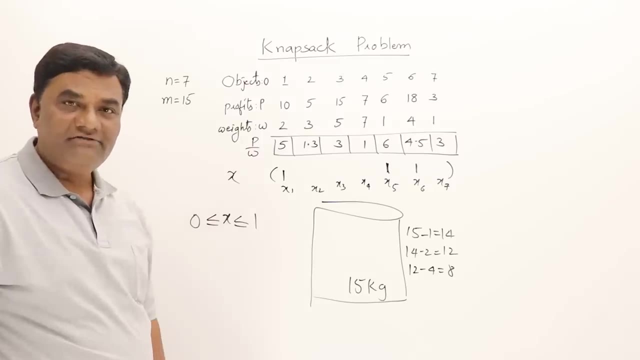 means all four kgs I will include. This is weight, Four kgs I will include. So this is 12 minus four is eight kg, Eight kg. I have included, right. So eight kg, Eight kgs are remaining. Now this is: 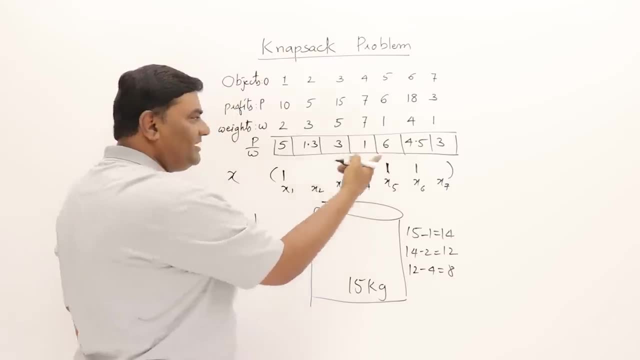 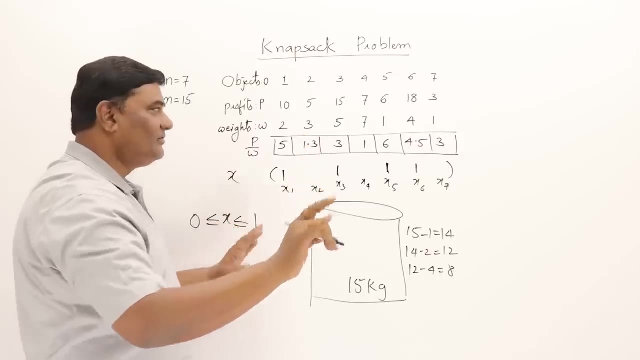 the next one. So I have three, three, These are two. I can pick up anyone, So I will select this object. So this is how many kgs? now, This is five kgs. Don't look at the weight. Don't look at the weight. I am selecting this one. This is giving profit by 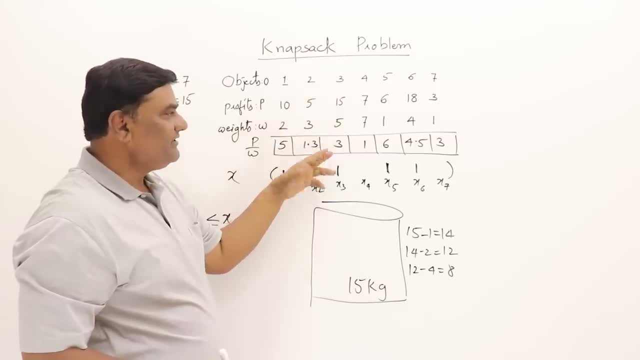 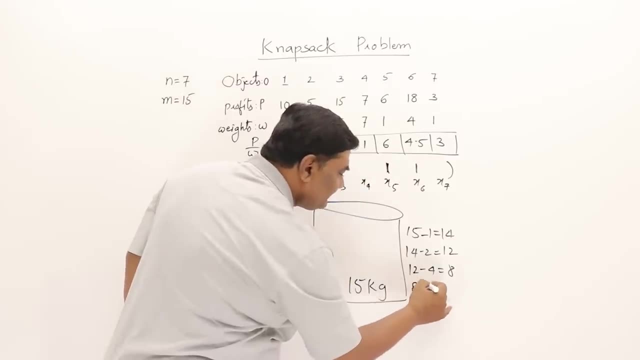 weight. So this is five kg and I'll be getting 15 profits. So the profit is same. only for both of them It is same, So I'll select this. So how many kgs are gone? Five kgs, So eight minus five, I am. 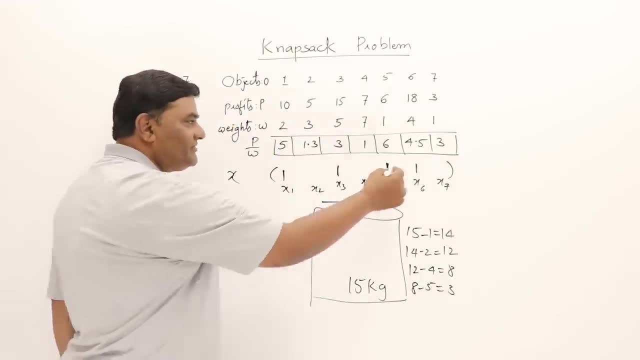 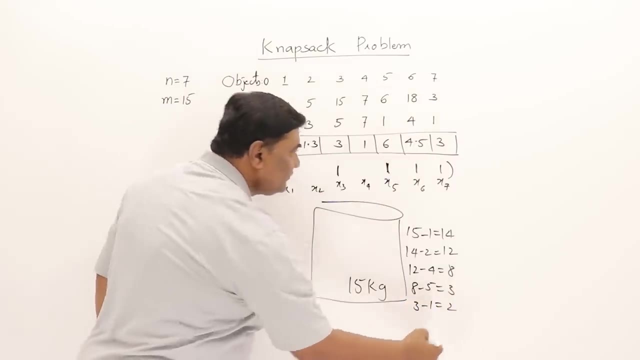 left with just three kgs in the bag. Now, next is which one? This one, So I will take this whole thing. So how many kgs? One kg, One kg. So three kgs are there Minus one. Now I am left with two kg. Now, which is the next one? 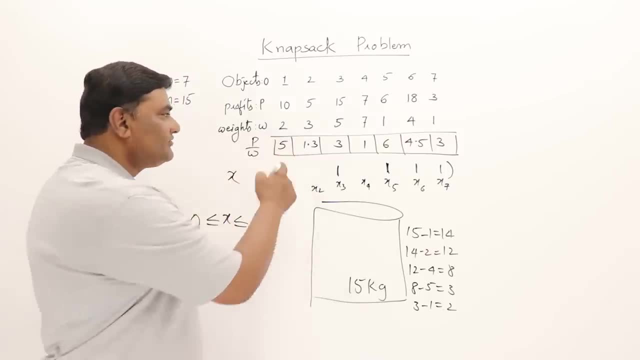 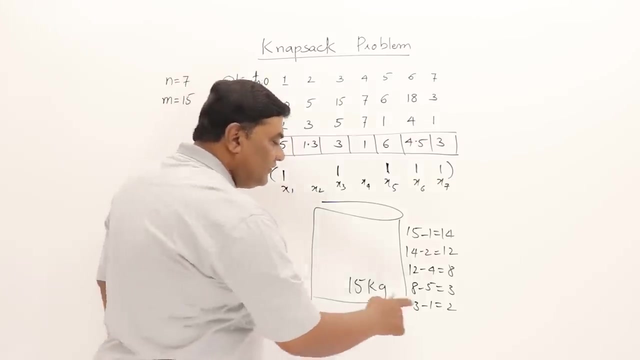 giving the profit. So this one, This one, So I will include this. But this is how many kg? Three kg. How much I have there? I have only two kgs remaining, So can I include all these three kgs there? No, I will be including only two kg there. So this is two minus two, Zero. It will become 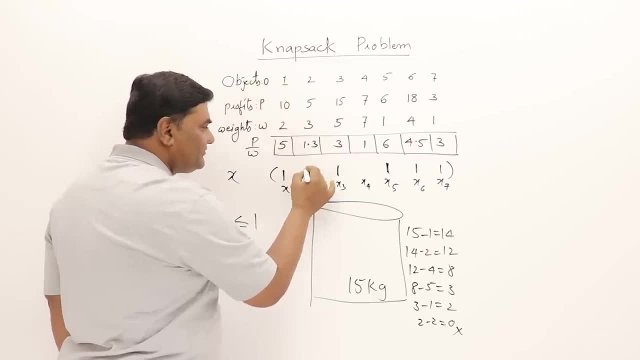 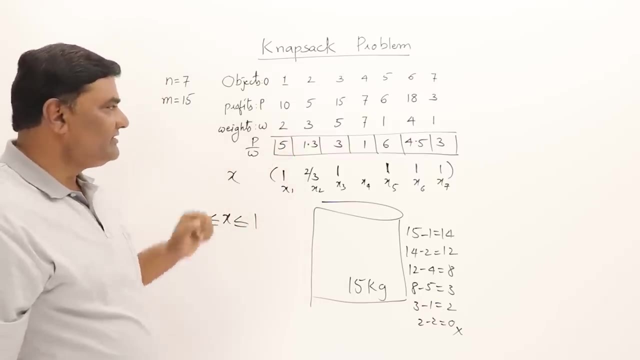 I am taking the full object. I am just taking two kg out of three. So this is two by three. Two by three, So I am taking the fraction of this object you said Already. I told you that these objects are divisible, So I am taking two kgs out of that. 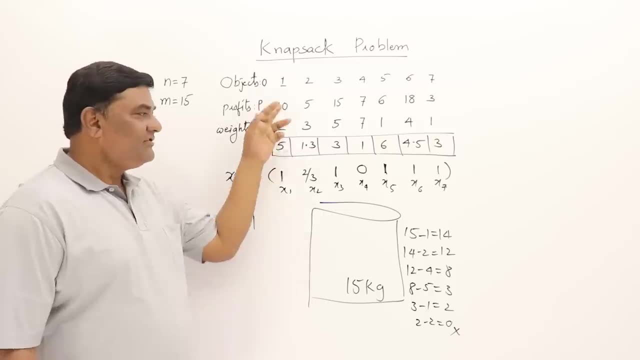 And what about this? This is not included. So I have a solution for this problem and this is the solution. This shows how I am going to include the objects, Which objects I should include, so that I get the maximum profit. Now I have to calculate the profit. 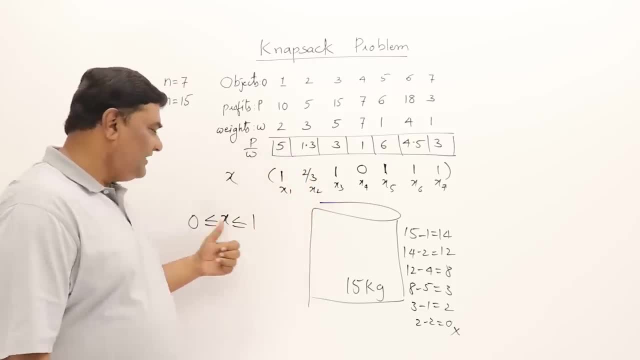 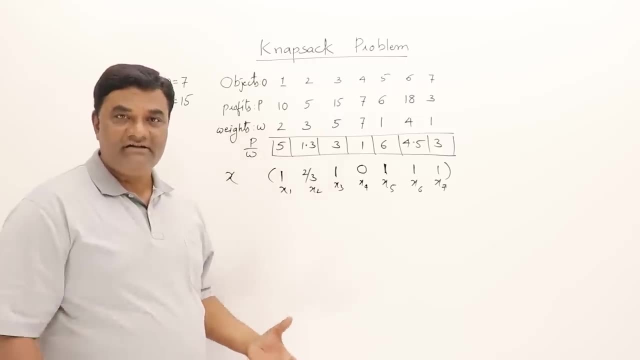 And find out how much it is. I have just written here the values from zero to one. Now I will see total, how much profit I get, and I will also verify the weight that I am getting- 15 kg only or not? Here I write these values, One with weight. 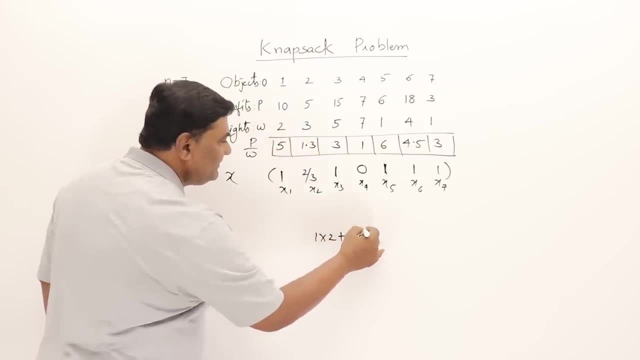 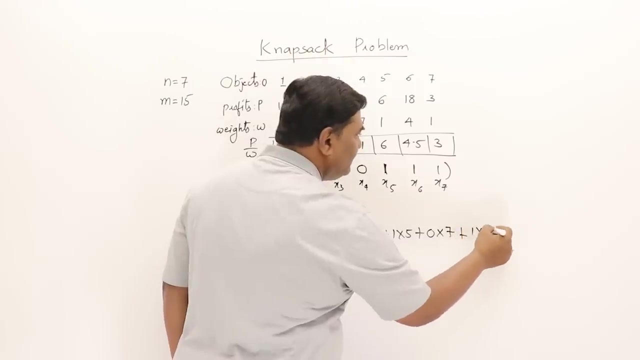 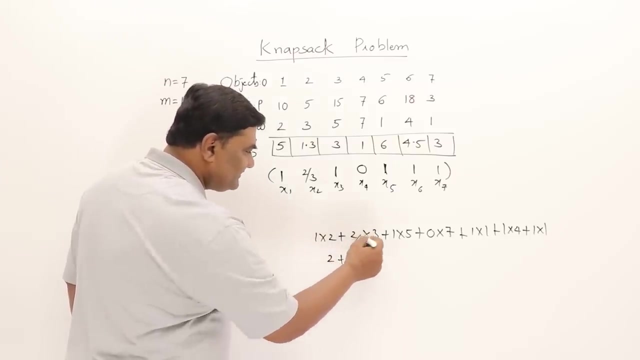 one into two plus two by three into this weight, three plus one into five plus zero into seven Plus one into one plus one into four kg plus one into one kg. If I take this, This is two plus this is two plus five plus zero plus one plus four plus one. 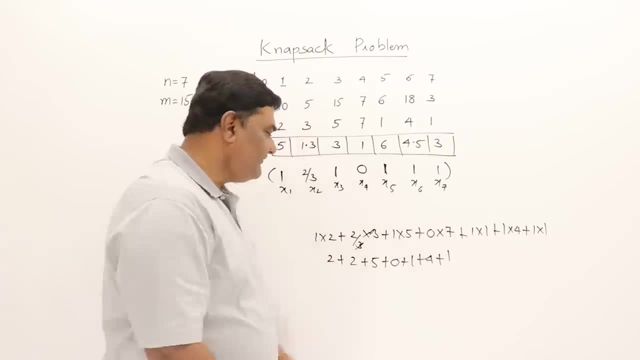 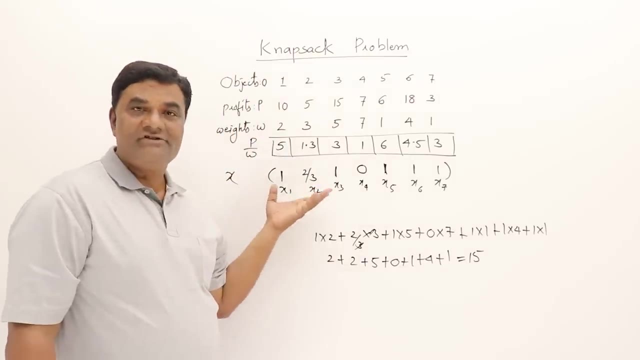 So this is nine, ten, fourteen plus one, fifteen. So, yes, the total weight is fifteen. only See, these are the x values. This is from zero to one, So that I am multiplying with weights. So what is this? Sum of the xi into weight i, and that is less than equal to fifteen. 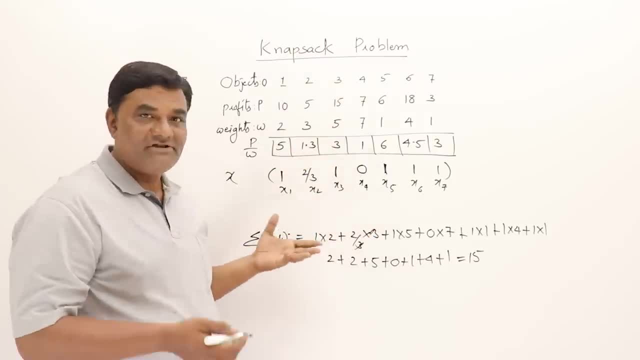 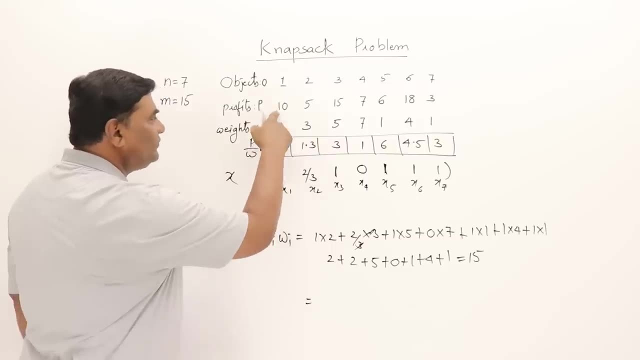 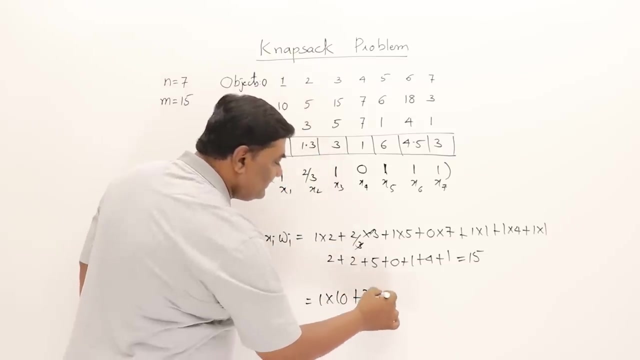 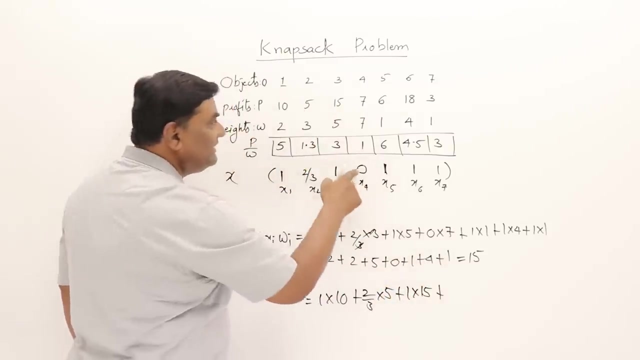 So I have found out the total weight. I was just subtracting. Now I am just verifying it. Now let me know the profit. So, for profit also, what I will do is one into ten plus two by three into five plus one into fifteen plus zero into seven. 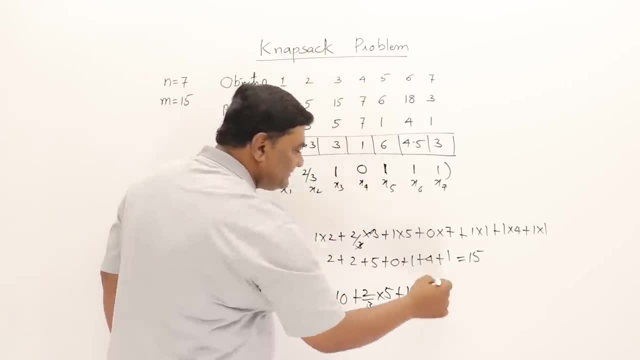 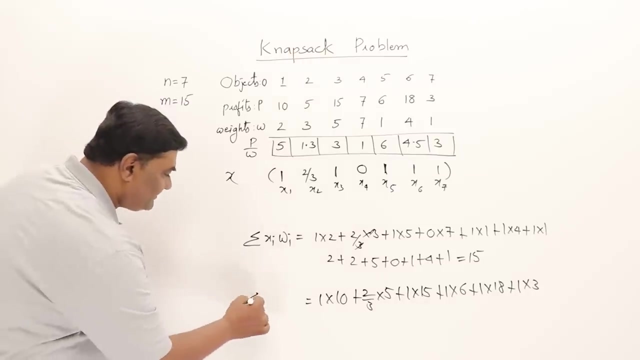 I will avoid writing it. Then. one into six plus one into eighteen, plus one into three, One into three, This is the profit. So this is nothing but summation of xi into pi. Every x value is multiplied with profit, So this is showing how much quantity I am taking x. 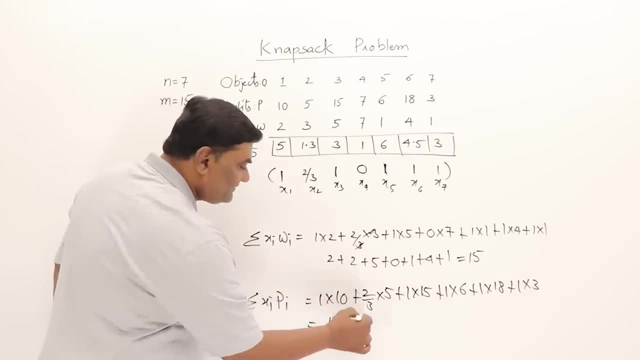 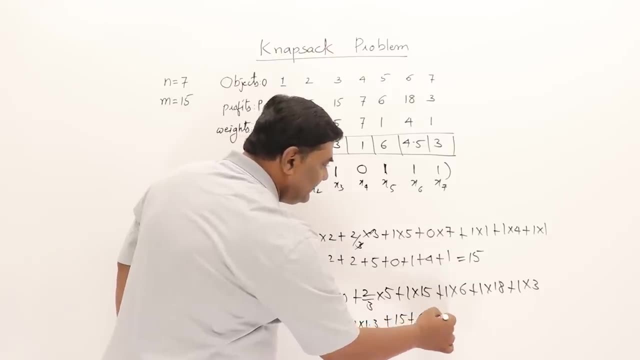 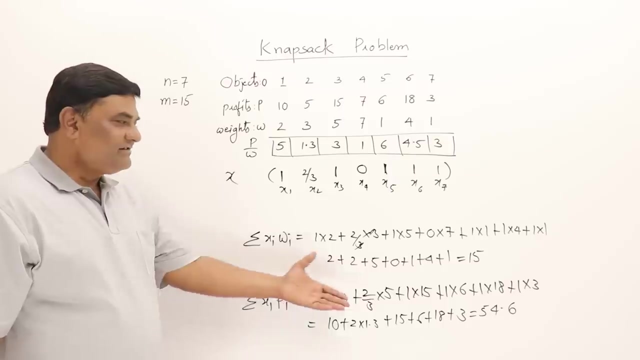 Now what is this total equal to? This is ten plus two into one point three, plus fifteen plus six, plus eighteen plus three, So this is fifty four point six. So that's it. Our total profit is fifty four point six and the total weight is fifteen. 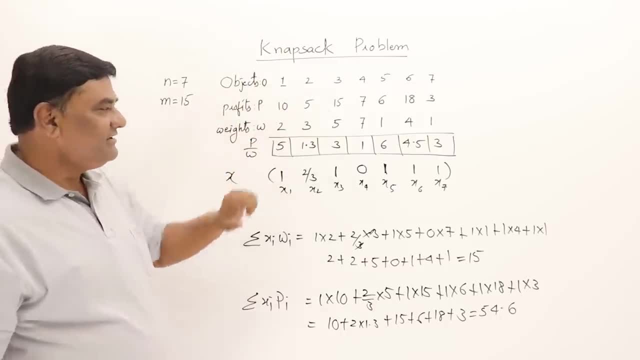 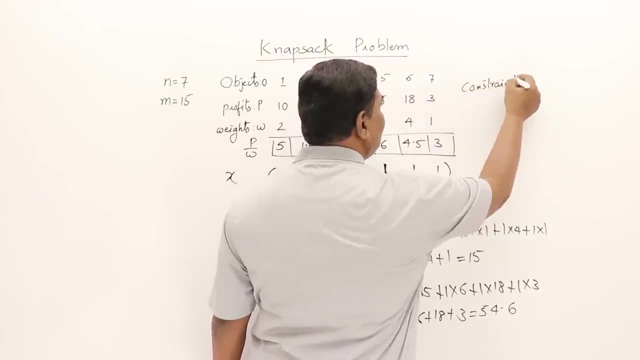 Once again, I will show you something here. See, these objects are given. Then what is the constraint given in the problem? The constraint is what Sum of the weights of the objects included in the bag should be less than equal to capacity of the bag? Yes, we have done it. 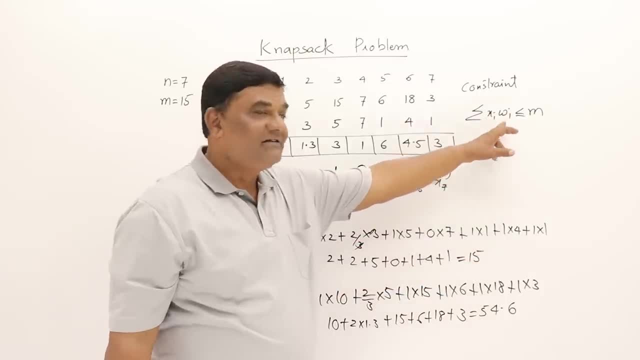 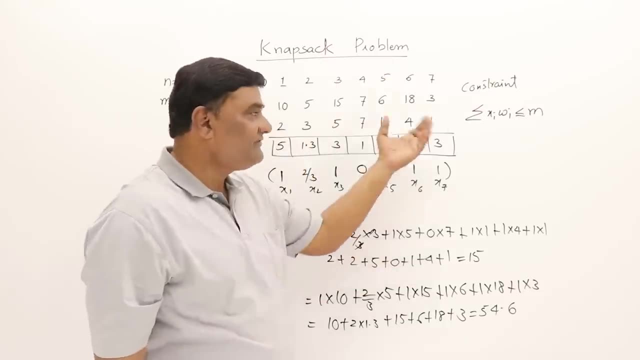 See, total weight should be less than equal to fifteen, and this is satisfied. This is the constraint given in the problem. So we have taken that solution which is satisfying the constraint. Yes, this solution is satisfying. So this is feasible And objective. is what 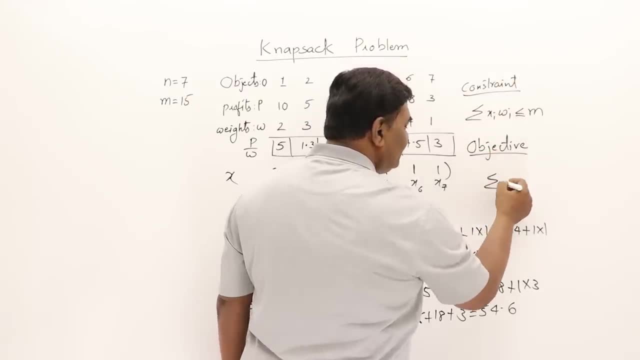 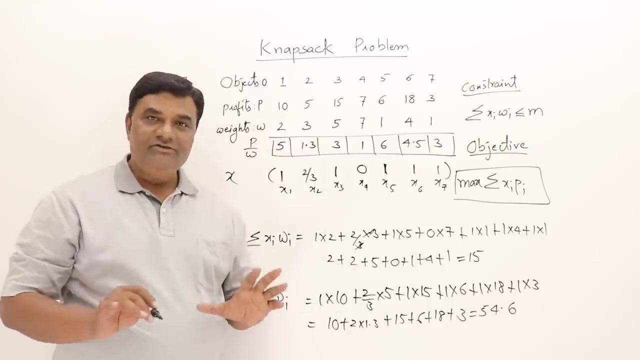 Objective is sum of the weights. profits of the objects that are included should be maximum. This is the objective Of a problem and we have achieved both. Now, quickly, I will explain you how we have followed the greedy method. Once again, I am explaining you See, the objects are given and the bag is given. 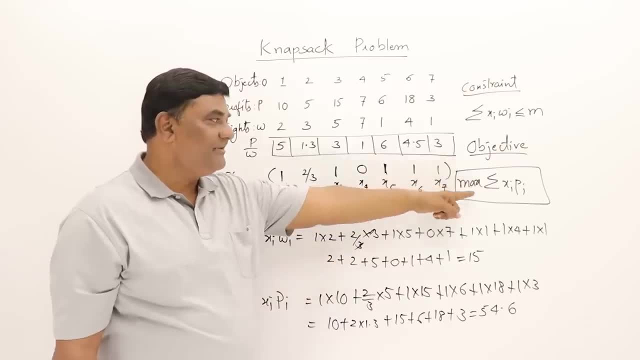 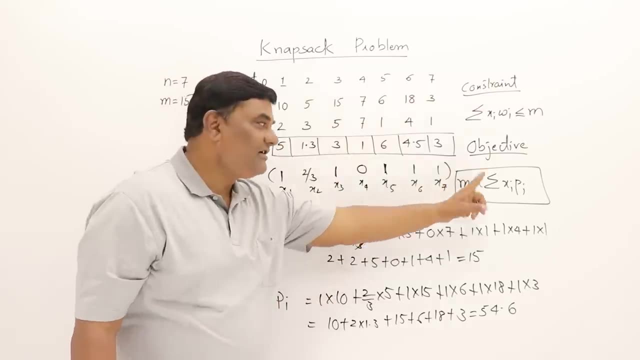 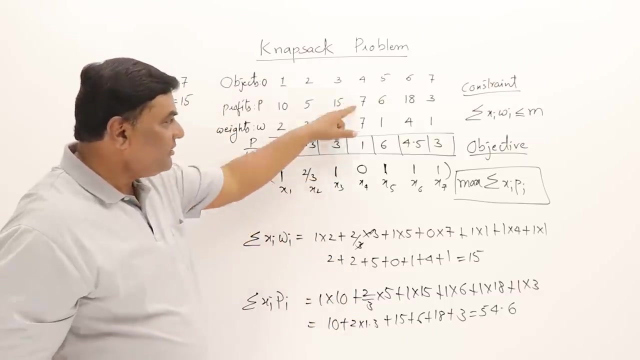 We have to include these objects in the bag such that the profit is maximum, but the total weight should not exceed that one. So we have to select some objects such that we guarantee that we are getting maximum profit. So we have decided the criteria of selection. Have we tried this object? No,